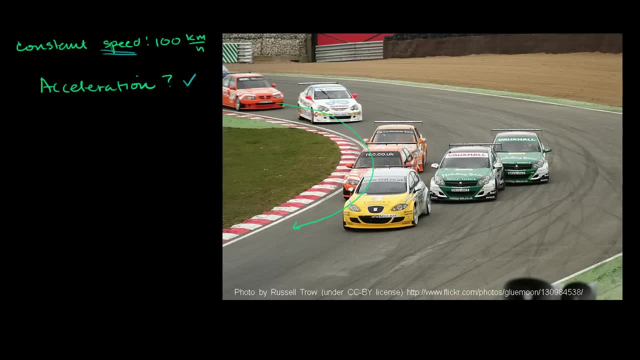 And to think about. let's take a top view of this thing And then I think it'll become a little bit clearer the difference between speed and velocity and why these things are accelerating. So if I were to take a top view of this racetrack, do my best. 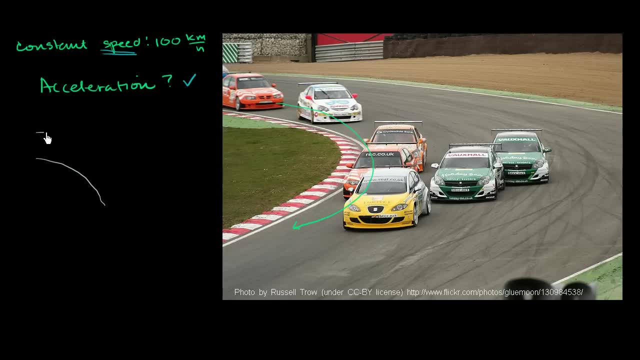 attempt to draw it, So it might look something like this. This is the top view. I could even draw this red and white, So red just to give you the idea. So this is the red and there's some white in between. 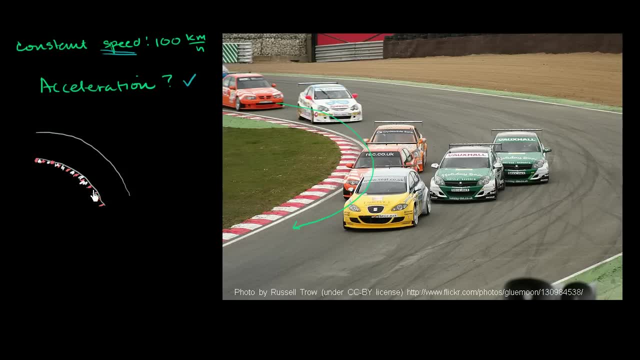 Obviously, I'm not drawing as many dividers as there are in the actual picture, but it gives you an idea of what I'm actually drawing. And then there's some grass out here. So there's some grass over here, and then there's some. 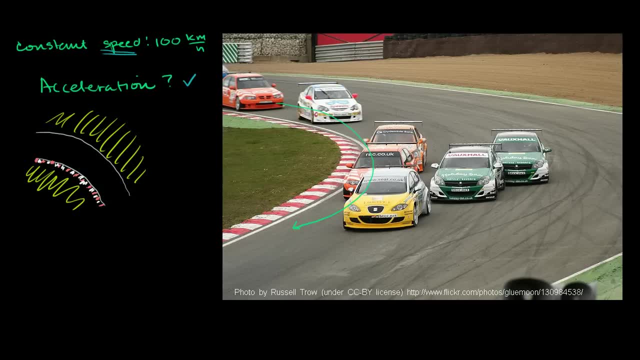 grass over here And let's focus on this orange car, this red car right over here. So where you say- And this is a top view, So this is its path- right over here, And we're saying it has a constant speed of 100. 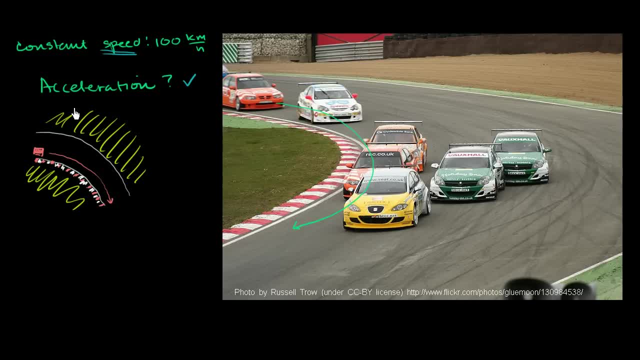 kilometers per hour. So if you think about its velocity, the magnitude of its velocity is constant. It is 100 kilometers per hour. But what is happening to the direction of the velocity? Remember, velocity is a vector quantity. It has magnitude and direction. 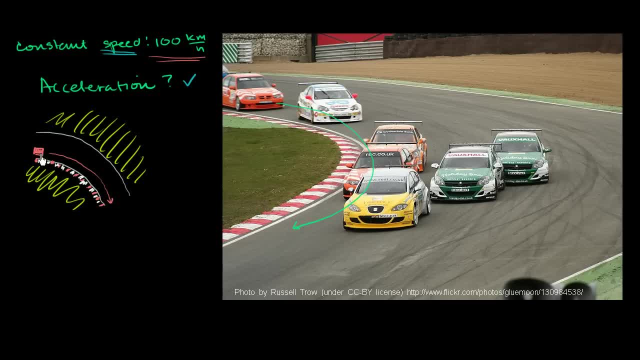 So up here at this one, it's starting to enter the curve, It's going in this direction, And you tend to show vectors by arrows like this, And what you do is the arrow is going in the direction of the velocity, in this case, 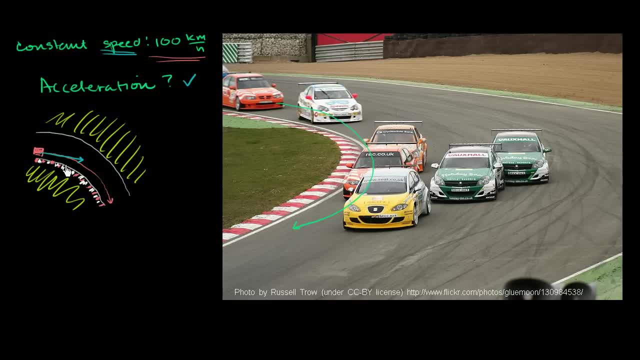 And normally you would draw. the length of the arrow shows what is the velocity, the magnitude of the velocity. I should say. So its velocity is constant. So the length of this arrow will always be constant, But as we see, its direction changes. 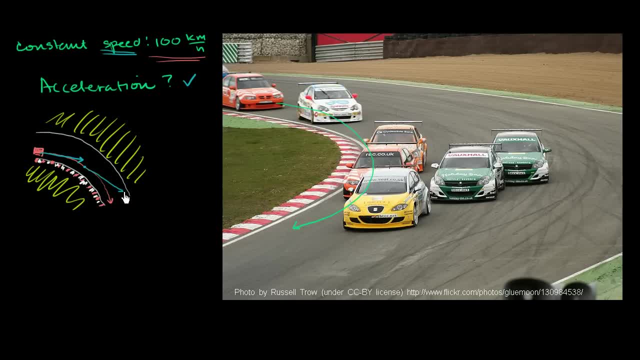 When it's halfway through the turn, it's not going in that same direction. It is now going in a different direction And when it comes to the bottom of the turn, it's going in a very different direction And it'll keep. 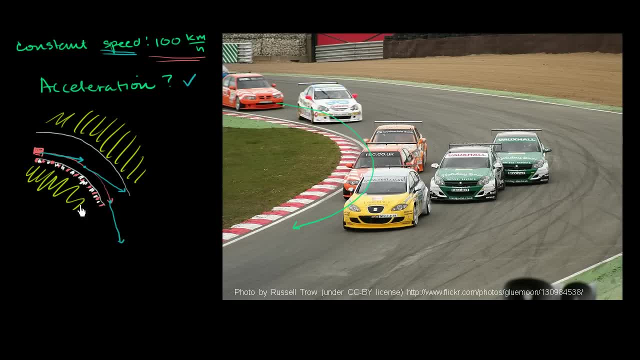 The direction keeps changing as long as it is turning. And I'm not going to go in the math here. We're going to wait for the math on this a little bit later. But remember, acceleration is a change in velocity over time. Acceleration is equal to a change in velocity over time.